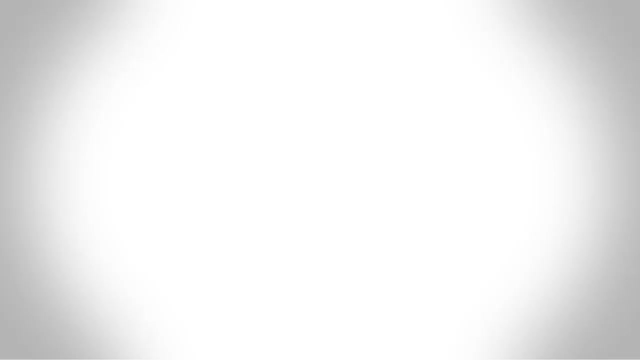 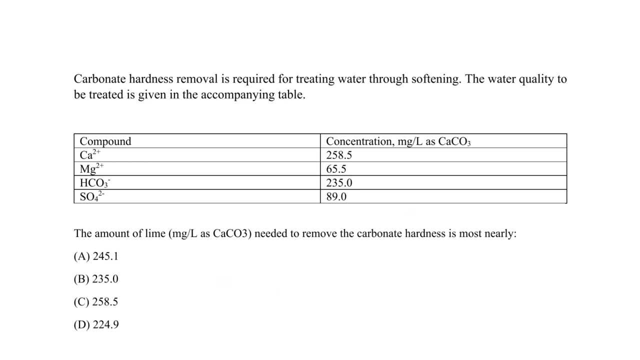 Okay, so now let's talk about water softening and how this relates to hardness, And we know we can expect a question about softening on our civil and environmental FE exams. So this relates more to environmental, but we have to understand it also for the civil section. 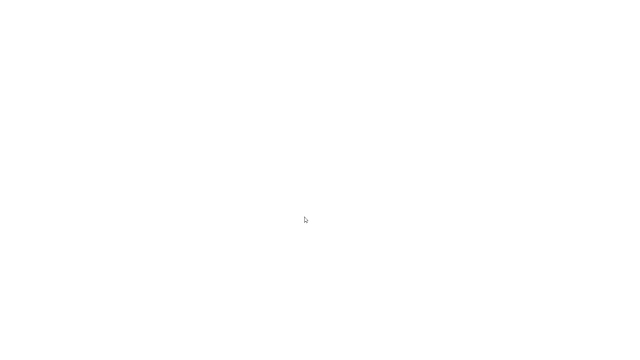 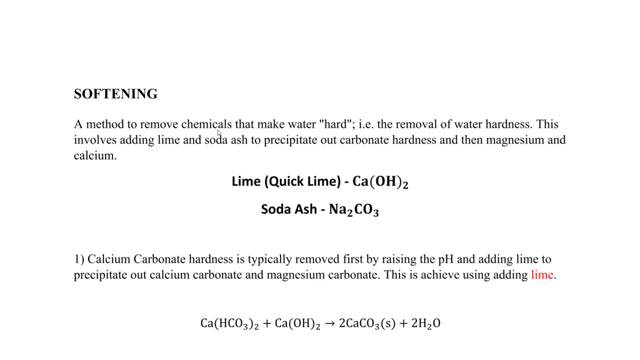 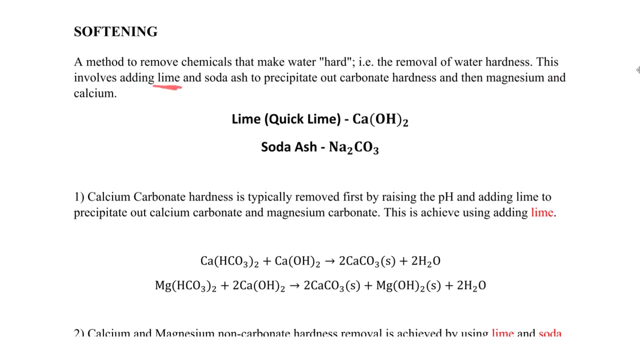 So we know here we're talking about softening and this relates to hardness. So this involves a method of removing the chemicals that make our water hard- Essentially, the removal of water hardness. So we know softening involves adding lime and soda ash, And what we're going to do. 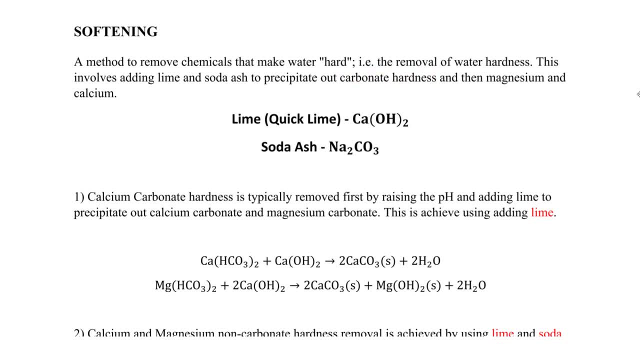 is precipitate out carbonate hardness first. That's what we'll do first, And this is generally done with lime. So we add lime in Our rapid mix basin And that's how we can remove this carbonate hardness. Then we can tree and precipitate out the magnesium and calcium, And this is a combination of lime. 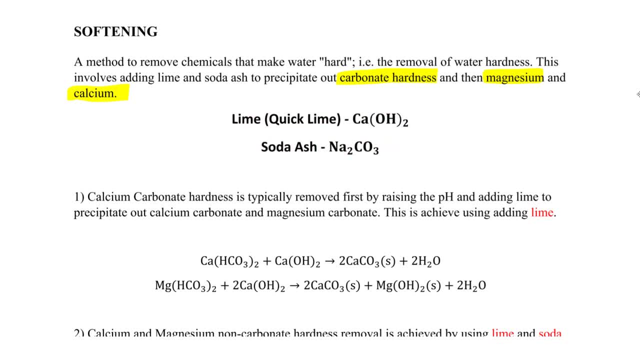 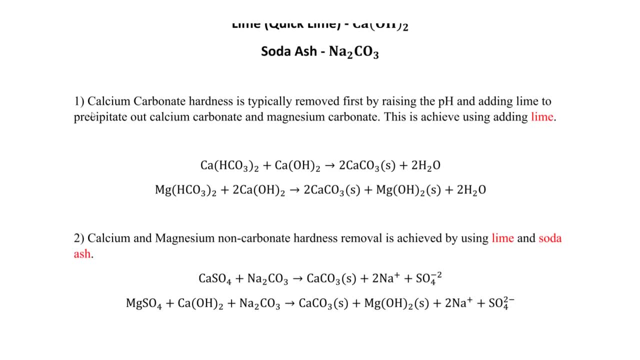 and soda ash. So these are the chemicals that are typically used. So lime is this and soda ash is the sodium carbonate. So we know step one here is to focus on the carbonate hardness. So we're going to be looking at the calcium carbonate hardness. 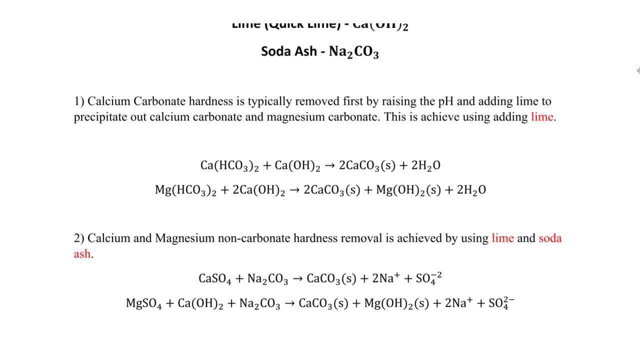 And we know this is removed first by raising the pH to around 10.3.. Then we add lime to precipitate out calcium carbonate and magnesium carbonate. So we do this by adding lime. So we know here, if we're looking at first calcium carbonate, We know we're focusing on calcium. 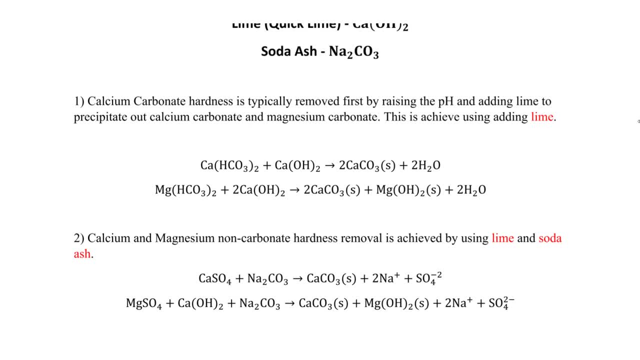 carbonate. So we want to precipitate out the calcium. So this is the calcium bicarbonate. Then we add the lime, So this is our lime. here. On the reactant side And on the product side we're going to get two calcium And this is. 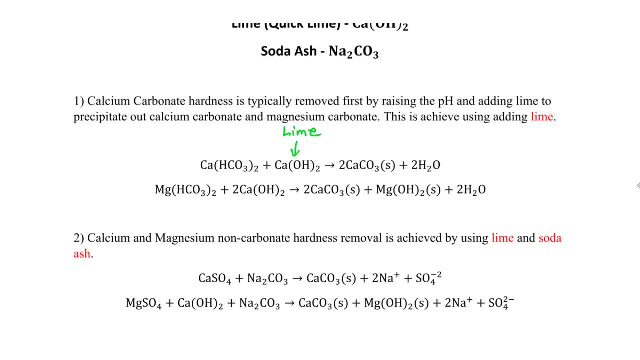 two, because we have one here and one here. One more of this, One more of this Gets us two of the on the right side, On the product side, And this is in the form of calcium carbonate as a solid. So that's for the calcium carbonate. For magnesium carbonate, we have a different. 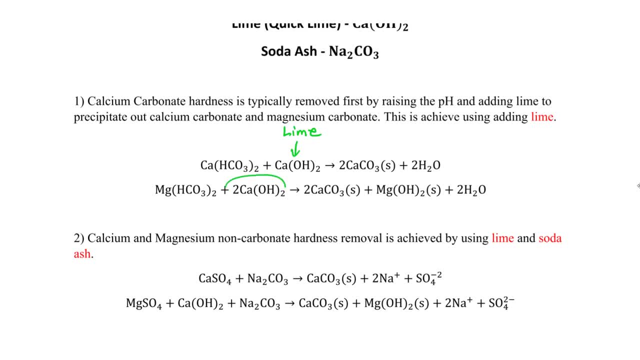 reaction. So we have the magnesium here. We add the lime, So this is still the lime And notice, here we precipitate out still two of calcium cause we have two here And we know we're going to also precipitate out the magnesium as well. We get that on the product side. So this: 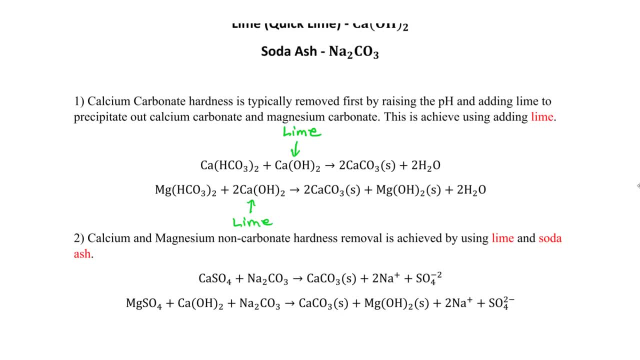 is for magnesium carbonate. This reaction And both of these reactions are given in the reference handbook. In the new reference handbook on page 341.. So let me write that this is on page 341.. in FE handbook, the newest one, handbook 10.0.1. so the latest one and this is under the lime soda. 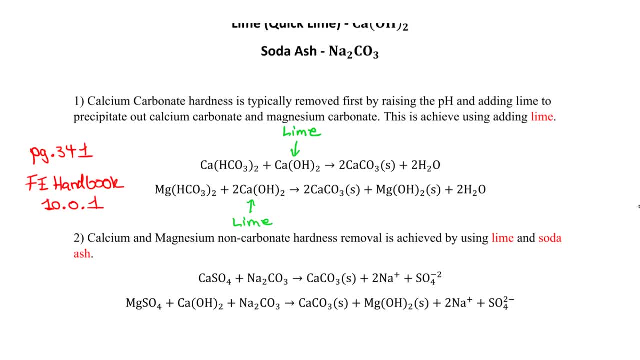 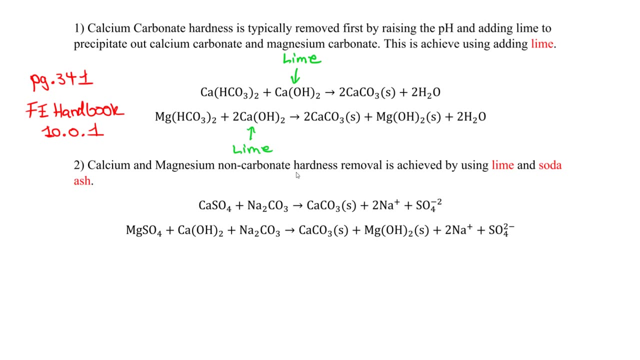 softening equations. this is for carbonate- the calcium carbonate hardness and magnesium carbonate. then that's for carbonate and that uses lime. notice how we use lime here, for the calcium and magnesium non carbonate hardness, which we have to also treat, is achieved by using the combination of lime and soda ash. so we use both lime and soda ash for the non carbonate hardness. so here we're. 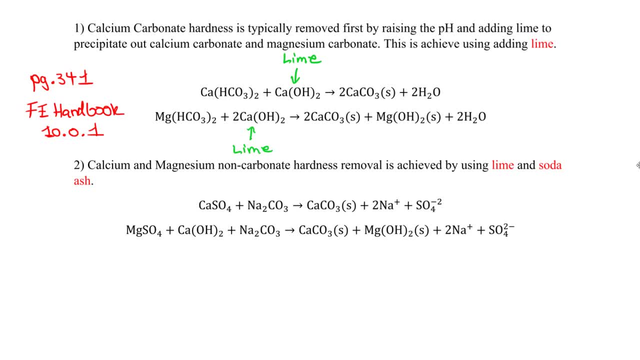 adding soda ash in this one. so this will be our soda ash and we know in the second reaction we're going to add both lime and soda ash. so we add lime here here and also we add soda ash, and this is specific to non-carbonate hardness. so these reactions 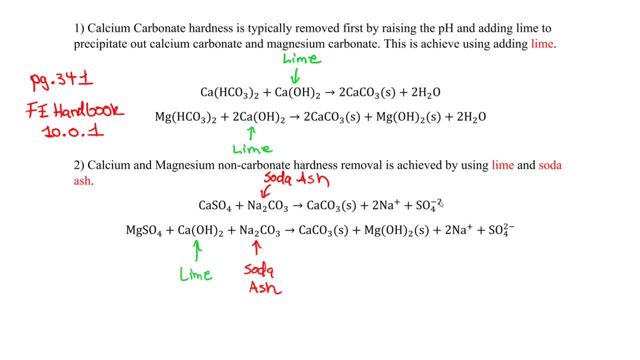 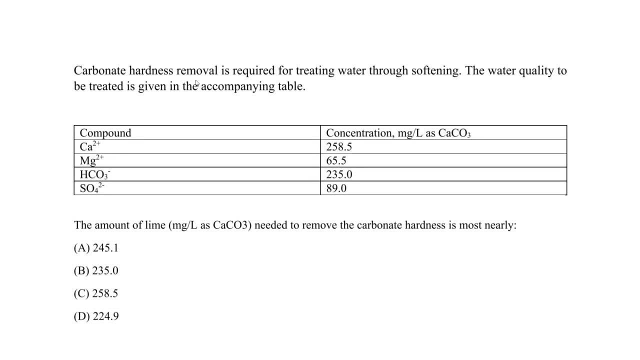 are also provided on the same page. so now let's, based on this understanding, let's do an fe type question real quick. we know here carbonate hardness removal is required for treating water through softening. the water quality to be treated is given in the table. so we have a table. 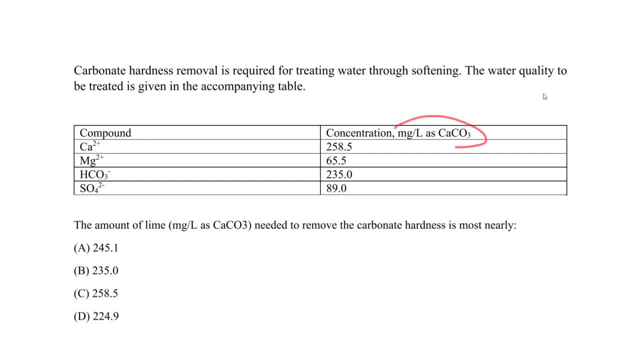 and we have our compounds and we're given the concentration as milligram per liter as calcium carbonate. so that's ice. they already converted that to us as a milligram per liter as calcium carbonate. so the question here is that amount of lime in milligram per liter is calcium carbonate? 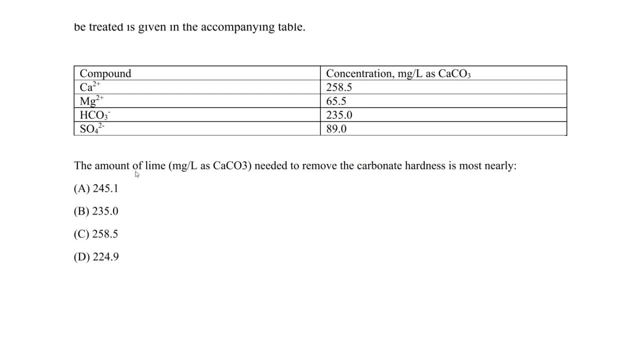 needed to remove the carbonate hardness is most nearly what. so what we're given is the data here. so this is given and what we want to find essentially is going to be the carbonate hardness. how much lime do we need lime do we need to treat to remove? essentially? 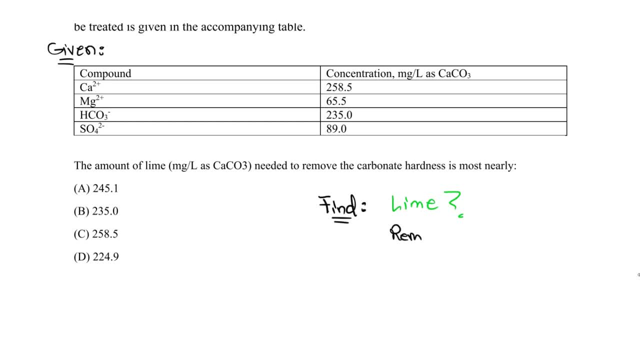 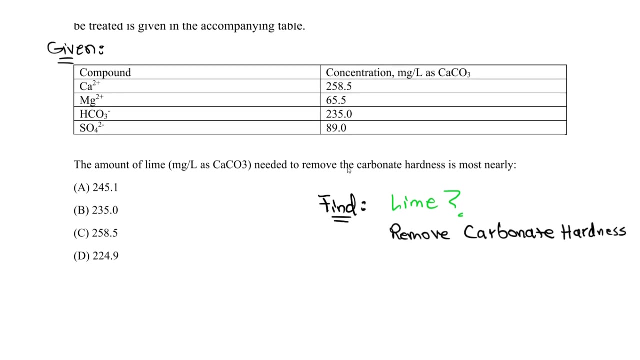 let me write: remove. and what we want to remove here is only the carbonate hardness. not, it's only so we're not looking at the carbonate hardness. so we're not looking at the carbonate hardness, we're only looking at carbonate hardness. so what do we do? I recommend first, let's draw our bar. 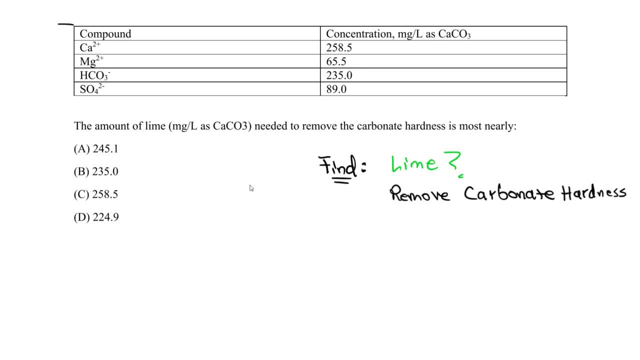 diagram and we know here we have calcium and it's gonna look something like that and we start at zero here and we have the magnesium here. so for calcium that concentration is 258- 0.5 and for magnesium it's going to be 65. so I take 258 plus 65.5, because 0 is here we're going. 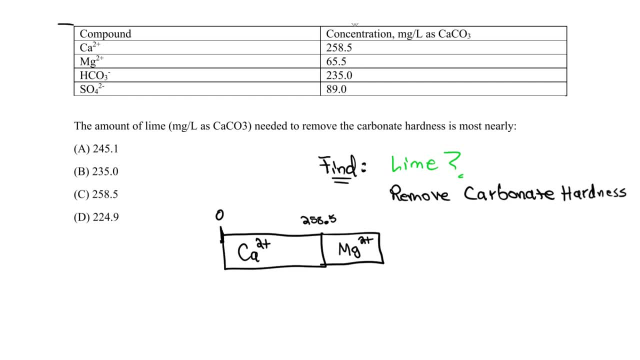 to the right. so you take the total 258 plus 65.5. we get this up to this point. we're going from left to right, we're increasing so that one should be 324 at this very end. so at the bottom we have the. we always place the bicarbonate and the. 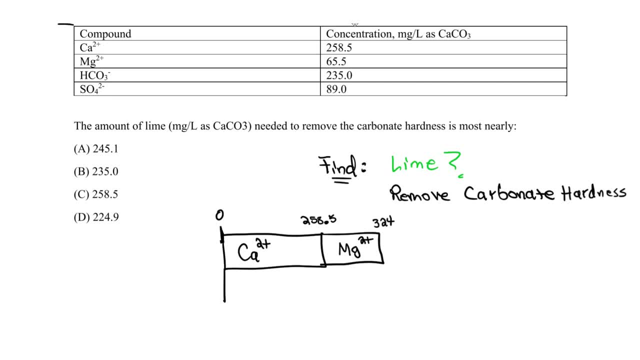 sulfate, so essentially the negative, and it's gonna be the 235. so we know it's before the 258, right, so it's gonna. I'll just say it's here, this is carbonate, and we know. then we have the sulfate and we take, we know, here is two thirty five point zero, then we just add the. 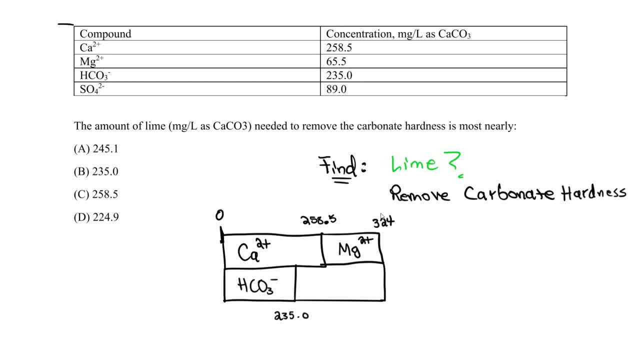 two, two thirty five plus eighty nine, and we'll get up to this point again: zeros. here we're going to the right, so there we should get three, twenty four, same as here. so this is the sulfate. so now we're looking at carbonate hardness. right, when you think of carbonate hardness, it always has. 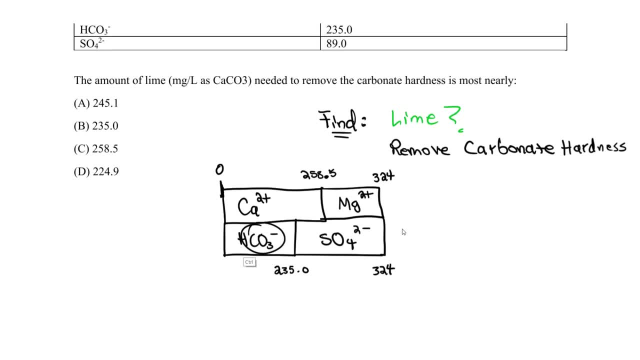 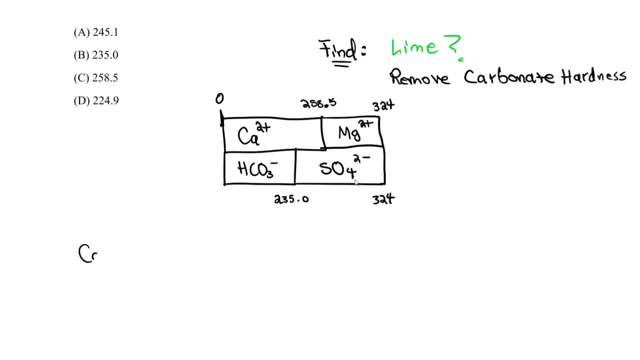 to have this carbonate right, this carbonate term, it has to have the alkalinity. so we know carbonate hardness. by definition, carbonate hardness, or CH, is going to be the minimum. it's the min of the total hardness, or so we're comparing the total hardness and the alkalinity. I'll just say a. 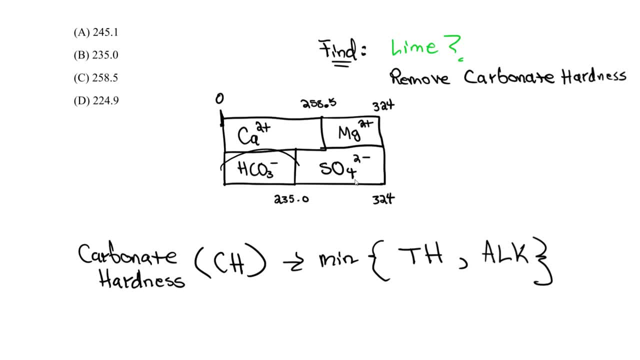 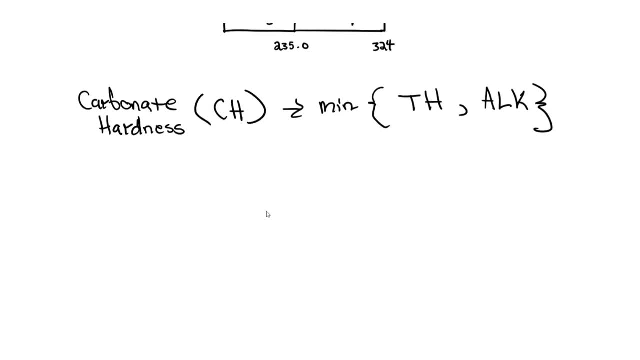 okay, and we know alkalinity is always going to be the bicarbonate ion. so alkalinity in this case is 235, so let's right there as two thirty five. so alkalinity is always the bicarbonate and this is two thirty five. and it can be meal gram per liter as calcium carbonate, which 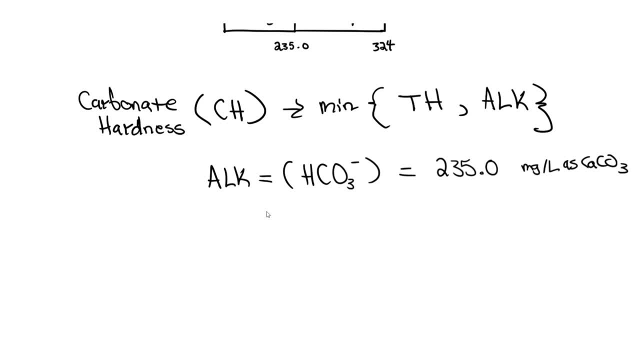 is the units we always want for alkalinity and a given to us. so we have that. what's the total hardness? the total hardness it's going to be the concentrations of the calcium and the magnesium. so let's add those together, the calcium and magnesium, which is also done for us, right? so we 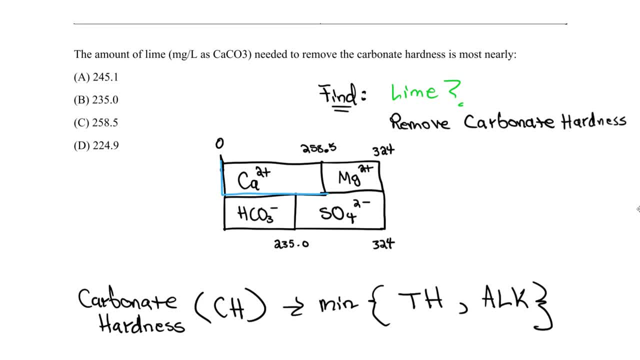 know that this is the total hardness. this portion here is indeed the total hardness. this is our th, so we just added the calcium and magnesium and get 324. this is our alkalinity. right, this will be our alkalinity. that's why we had. it's good that you draw a bar diagram, because you can visually see the total. 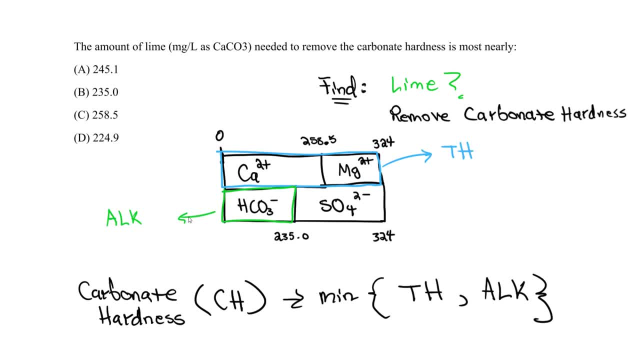 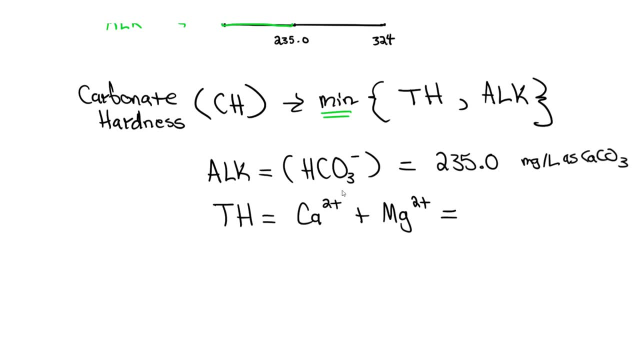 hardness is bigger than the alkalinity. that means we have to take the minimum of those. so which one is the minimum of the alkalinity, and which one is the minimum of the alkalinity, and which one do we do? we pick, obviously the alkalinity. so let me just write the total hardness here, which is 324, right. so 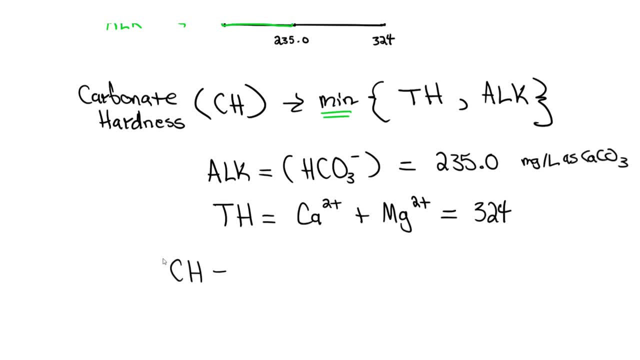 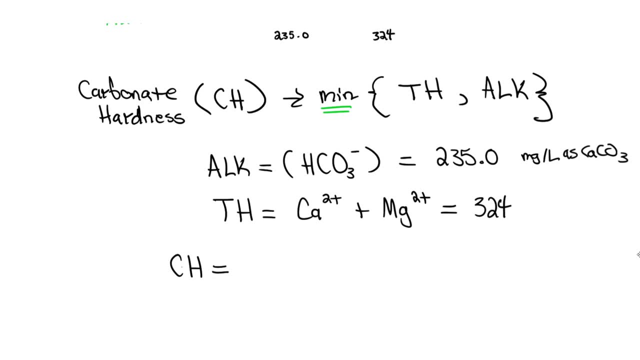 the carbonate hardness. our CH is going to be. what is that alkalinity? because we have to take the minimum. so that's going to be our carbonate hardness and it's just the alkalinity value. so we take 235.0 milligram per liter as one. 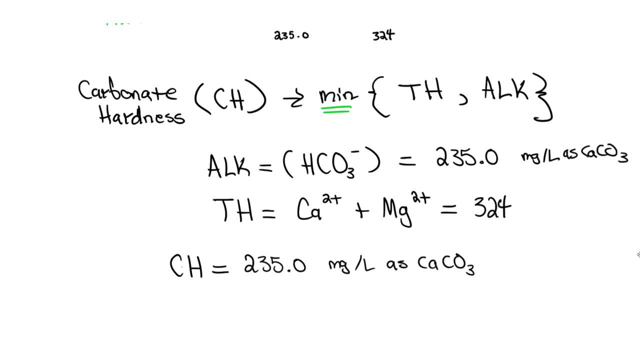 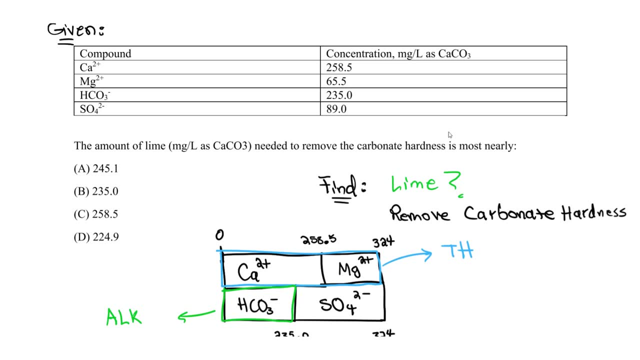 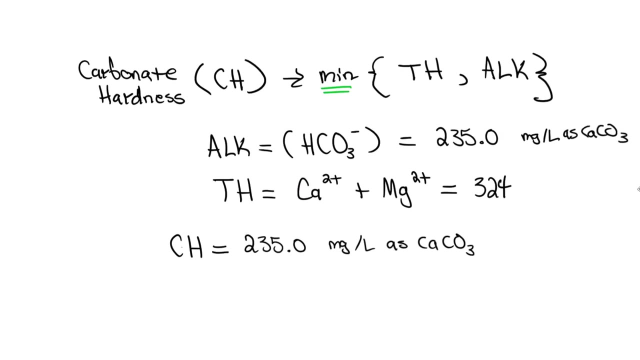 as calcium carbonate. So this is the carbonate hardness. and this question asks us: how much lime do we need? So, essentially, we are only treating for carbonate hardness. so the amount of lime we need is just this value. So this is our answer. so the lime needed here is going. 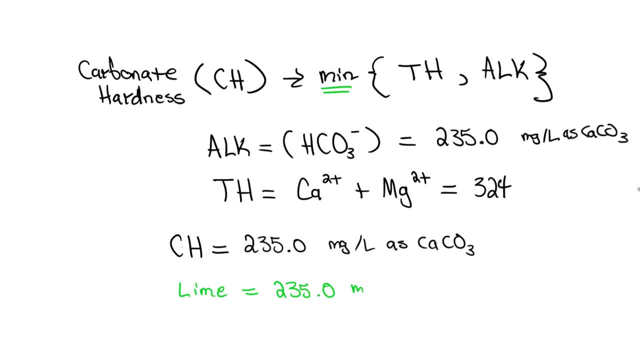 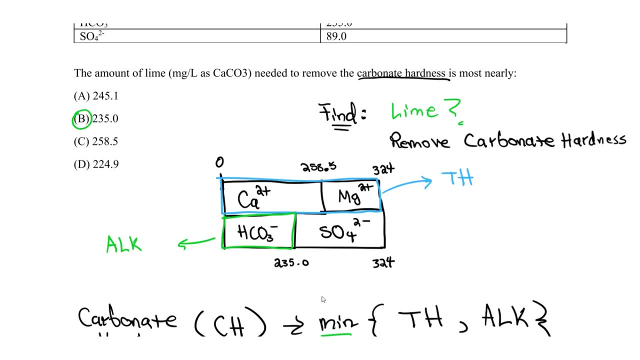 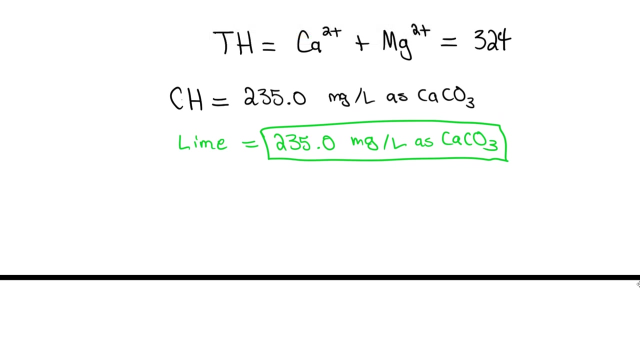 to be 235.0 mg per liter as calcium carbonate. So this is our answer And if we look at our choices, it should be b. One last thing is we have the carbonate hardness. lets say we want the noncarbonate hardness. so the definition of that NCH is going to equal to the total. 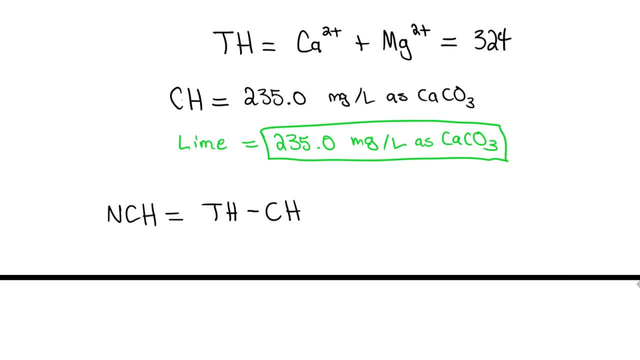 hardness minus carbonate hardness. so the non-carbonate hardness is going to equal what's the total hardness? It's 324 minus the carbonate hardness, which is 235, and if you do the math for that, you should get around 89.. So this is milligram per liter as calcium carbonate. 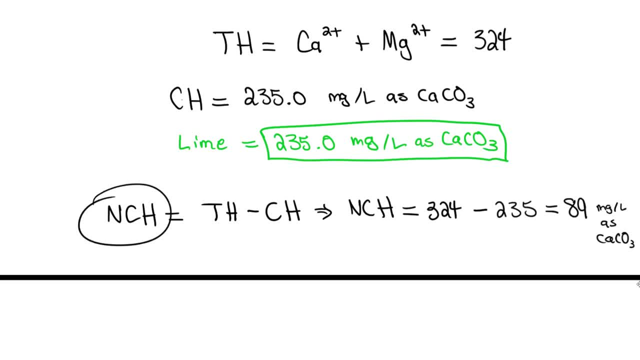 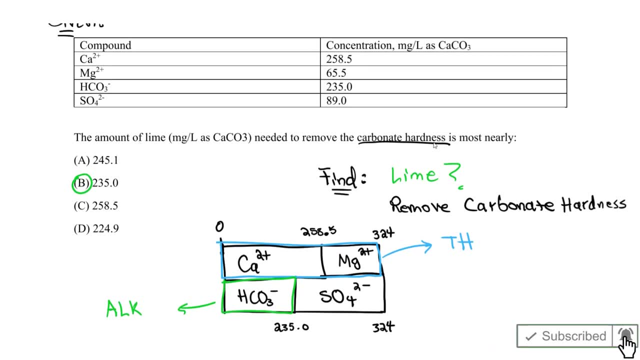 So that's just the extra note. this is the non-carbonate hardness, But our correct answer for this question should be B, the amount of lime needed to remove, just the carbonate hardness.